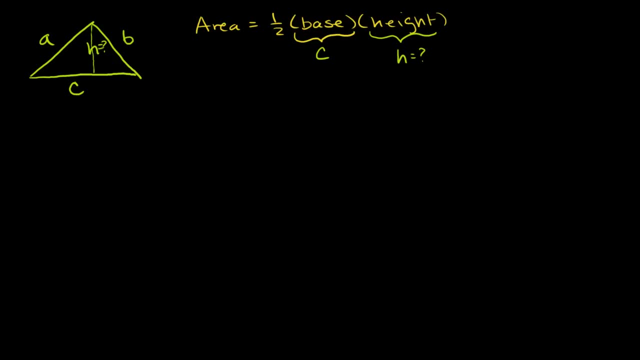 and figure out the area of this triangle. So we already labeled this as h. Let me define another variable here. Let me define. this is a trick you'll see pretty often in geometry. Let me define: this is x, and if this is x in magenta, then 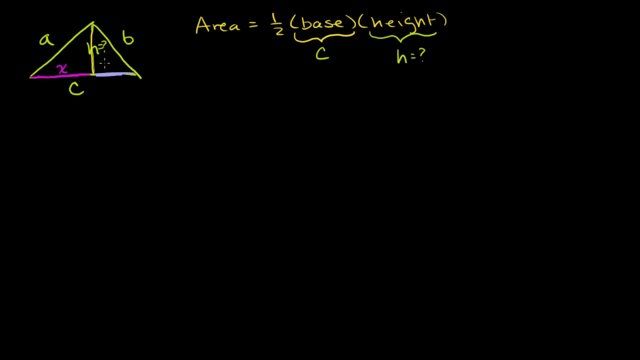 in this bluish, purplish color, That would be c minus x. right, This whole length is c, The whole base is c. So if this part is x, then this part is c minus x. And what I could do now? because since these are both, 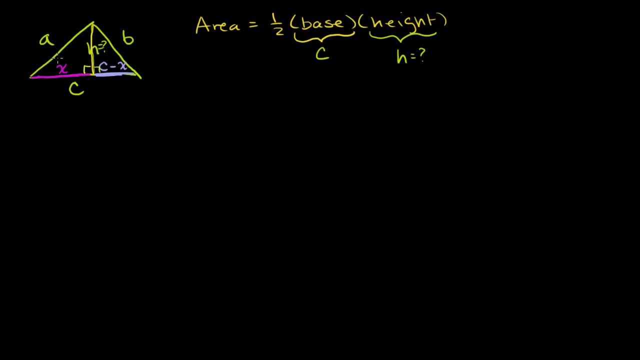 right angles and I know that because this is the height, I can set up two Pythagorean theorem equations. First, I could do this left-hand side and I can write that x squared plus h squared is equal to h squared a squared. 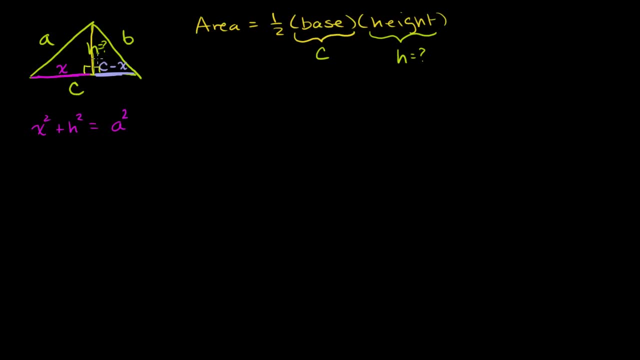 That's what I get from this left-hand triangle, And then from this right-hand triangle I get c minus x squared plus h squared is equal to b squared. So I'm assuming I know a, b and c. So I have two equations with two unknowns. 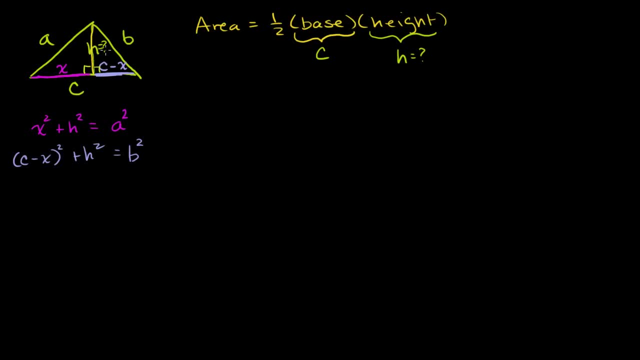 The unknowns are x and h, And remember, h is what we're trying to figure out, because we already know c. If we know h, we can apply the area formula. So how can we do that? Well, let's substitute for h to figure out x. 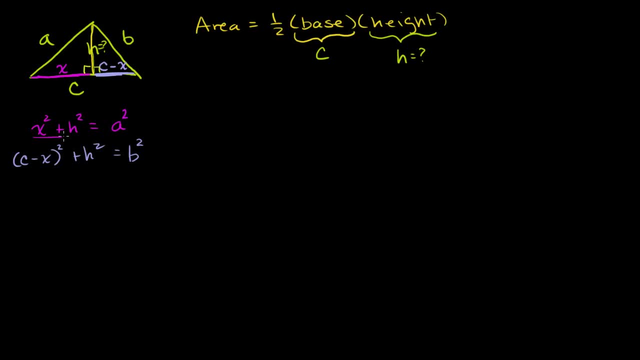 When I say that, I mean let's solve for h squared here. If we solve for h squared here, we just subtract x squared from both sides. we can write that h squared is equal to a squared minus x squared, And then we could take this information and substitute it. 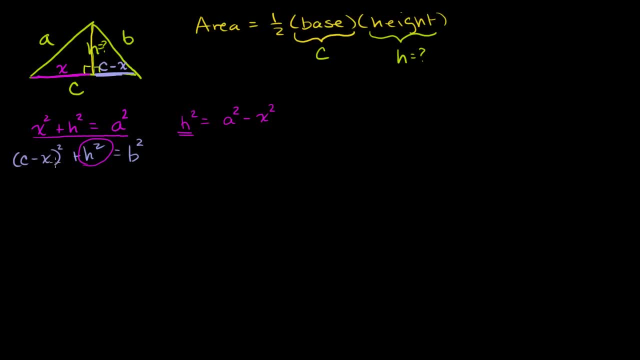 over here for h squared. So this bottom equation becomes c minus x squared plus h squared, h squared. we know from this left-hand side equation h squared is going to be equal to, so plus. I'll do it in that color. a squared minus x squared is equal to b squared. 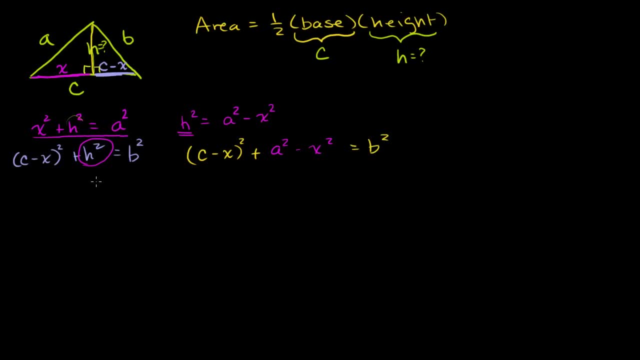 I just substituted the value of that in here the value of that in there. Now let's expand this expression out: c minus x minus x squared, that is c squared minus 2cx plus x squared, and then we have the minus a. sorry, we have the plus a squared plus a squared minus x squared equals b squared is equal to b squared. we have an x squared and a minus x squared there. so those cancel out. those cancel out. 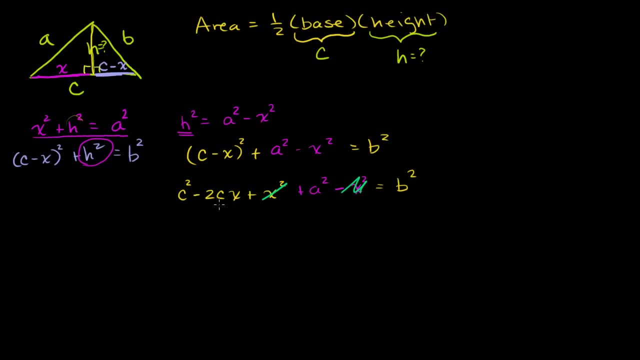 and let's add the 2cx to both sides of this equation. so now our equation would become: c squared plus a squared plus a squared. I'm adding 2cx to both sides, so you add 2cx to this, you get 0, is equal to b squared plus 2cx. all I did here is I cancelled out the x squared and then I added 2cx to both sides of this equation. 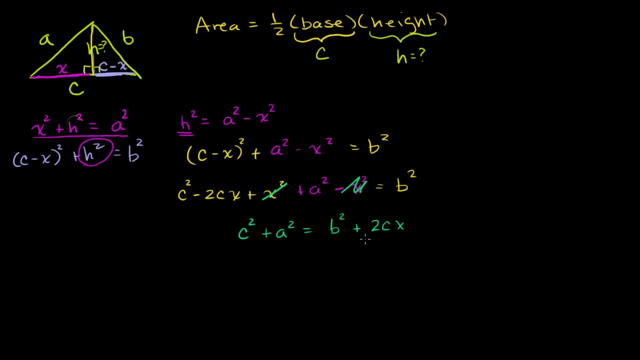 my goal here is to solve for x, and once I solve for x, then I can solve for a, I can solve for h and apply that formula now to solve for x. let's subtract b squared from both sides, so we'll get c squared plus a squared minus b squared is equal to 2cx, and then if we divide both sides by 2c, we get c squared plus a squared minus b. squared over 2c is equal to x. 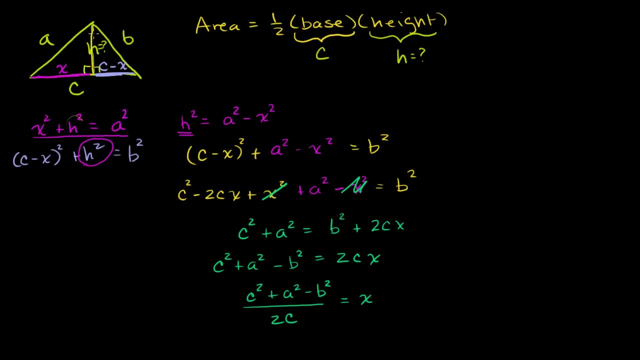 we've just solved for x. Now our goal is to solve for the height, so that we can apply 1 half times base times height. so to do that, we go back to this equation right here and solve for our height. 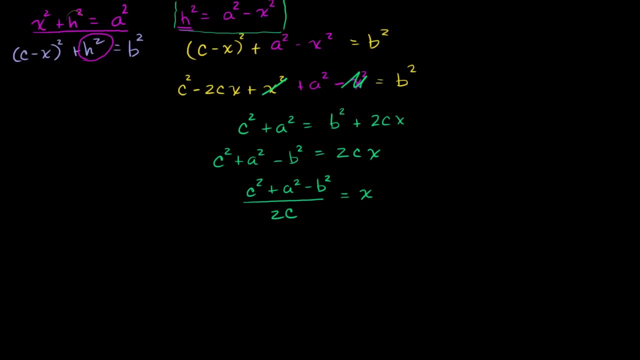 so let me scroll down a little bit. we know, we know that our height squared, that our height squared is equal to a squared, a squared minus x squared. well, instead of x, just writing x squared, let's substitute here, so it's minus. 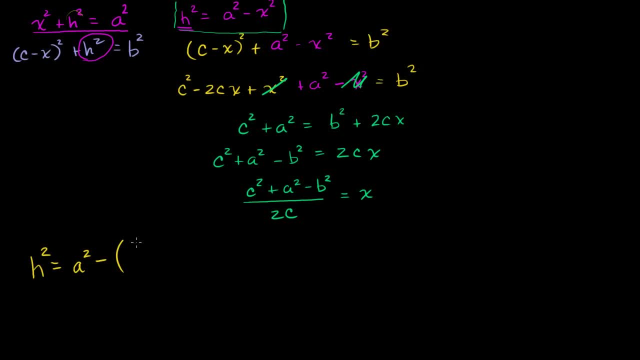 x squared. x is this thing right here. so c squared plus a squared minus b squared over 2c squared, this is the same thing as x squared. we just solved for that. so h is going to be equal to h is going to be equal to the square root of all this business in there. I'll switch the colors of a squared minus. 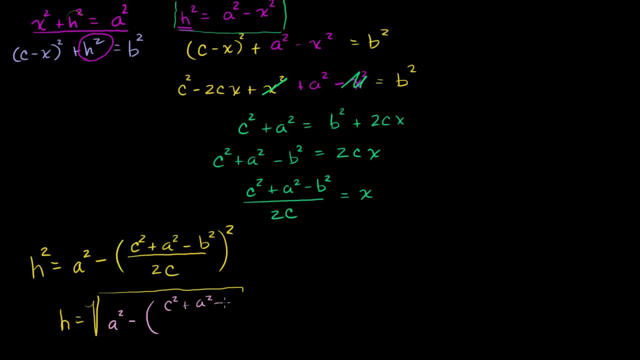 c squared plus a squared minus b squared- all of that squared actually. let me make it a little bit neater than that, because I don't want to the square root. the square root. make sure I have enough space of a squared minus all of this stuff squared. we have c squared plus a squared minus b squared- all of that squared actually. let me make it a little bit neater than that, because I don't want to the square root, the square root. make sure I have enough space of a squared minus all of this stuff squared. we have c squared plus a squared minus b squared- all of that squared actually. let me make it a little bit neater than that, because I don't want to the square root, the square root. make sure I have enough space of a squared minus all of this stuff squared. we have c squared plus a squared minus b squared- all of that squared actually. let me make it a little bit neater than that, because I don't want to the square root. 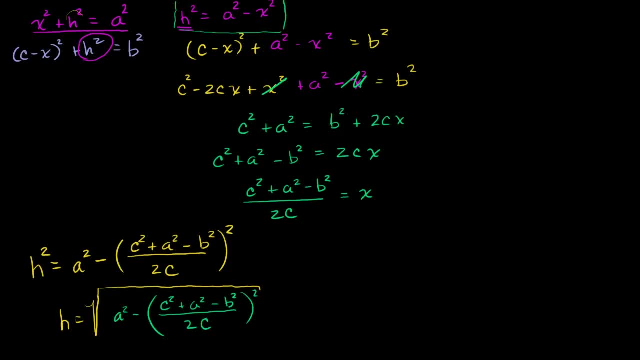 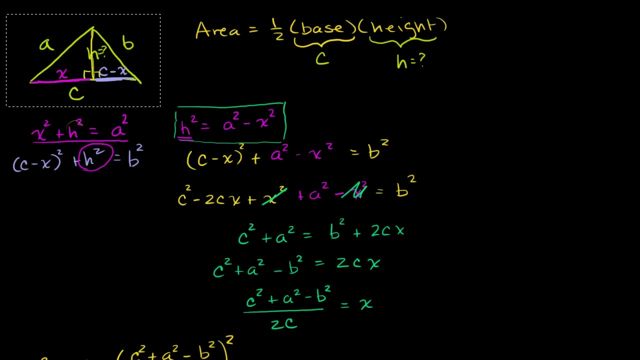 that over 2c. That is the height of our triangle, the triangle that we started off with up here. Let me copy and paste that, just so that we can remember what we're dealing with. Let me copy it and then let me paste it down here. 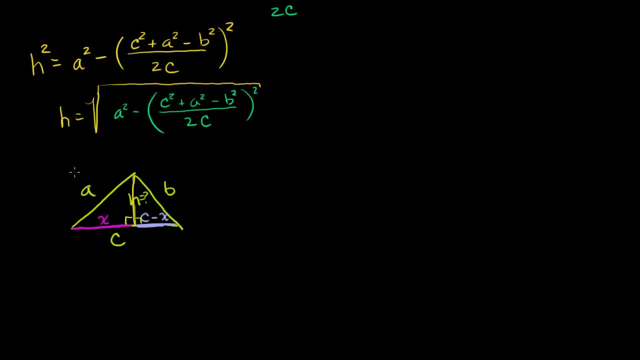 So we know what the height is. It's this big convoluted formula: The height in terms of a, b and c is this right here? So if we wanted to figure out the area, the area of our triangle, I'll do it in pink. 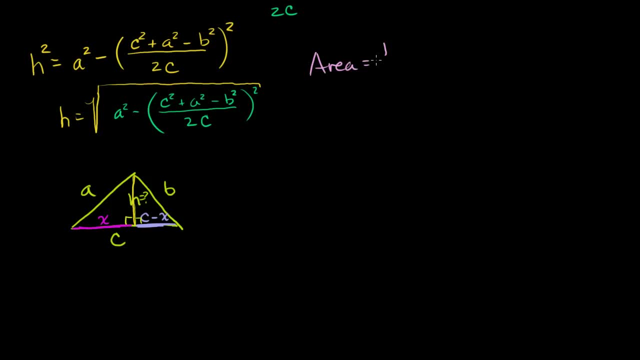 The area of our triangle is going to be 1 half times our base. our base is this entire length, c times c times our height, which is this expression right here. Let me just copy and paste it instead of so copy and paste. 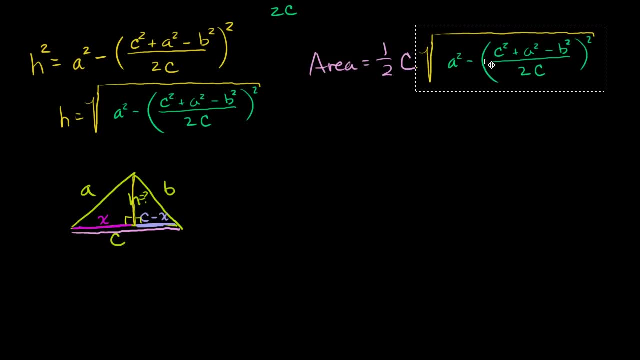 So times the height. So this now is our expression for the area. Now you're immediately saying, gee, that doesn't look a lot like Heron's formula. And you're right, It does not look a lot like Heron's formula. 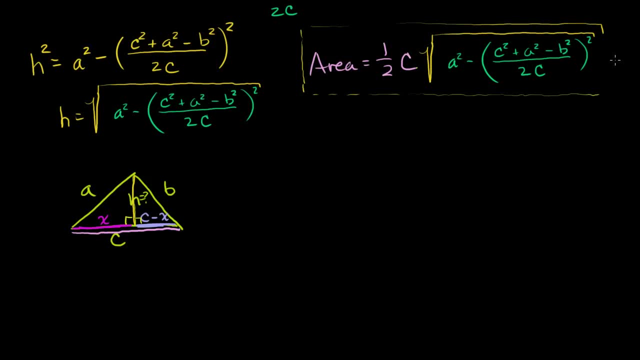 But what I'm going to show you in the next video is that this essentially is Heron's formula. This is a harder to remember version of Heron's formula. I'm going to apply a lot of algebra to essentially simplify this to Heron's formula. 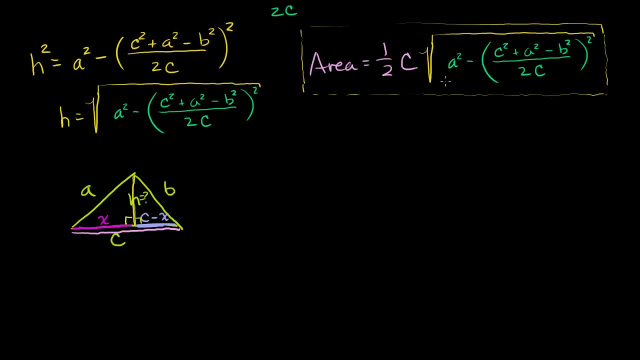 But this will work If you could memorize this. I think Heron's is the best way to do this. Heron's is a lot easier to memorize, But if you can memorize this and you just know a, b and c, 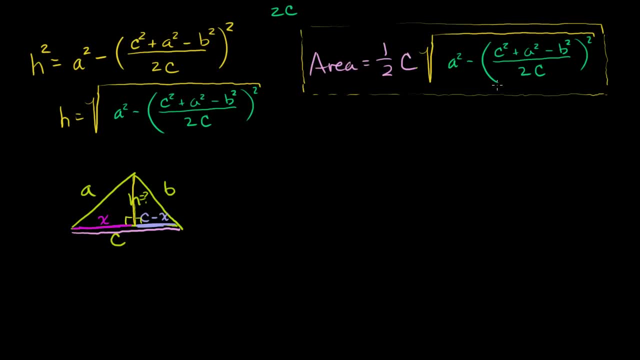 you apply this formula right here and you will get the area of a triangle. Well, actually, let's just apply this, just to show that this at least gives the same number as Heron's. So in the last video we had a triangle that had sides 9,, 11,. 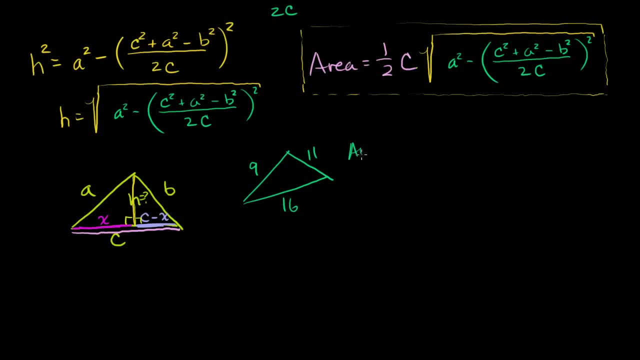 and 16, and its area, using Heron's, was equal to 18 times the square root of 7.. Let's see what we get when we apply this formula here. So we get: the area is equal to 1 half times 16 times the. 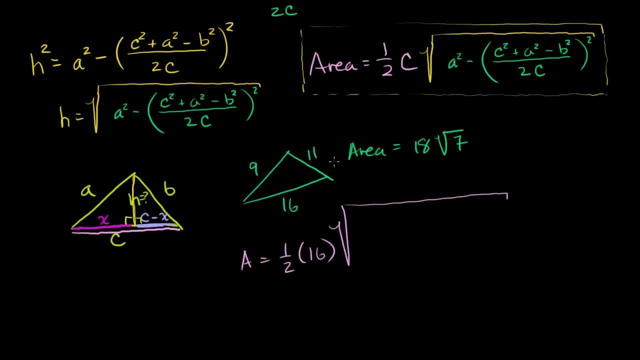 square root of a squared, That is 81 minus. let's see c squared is 16.. So that's 256.. Plus a squared, that's 81, plus 81, minus b squared, So minus 121.. All of this stuff is squared. 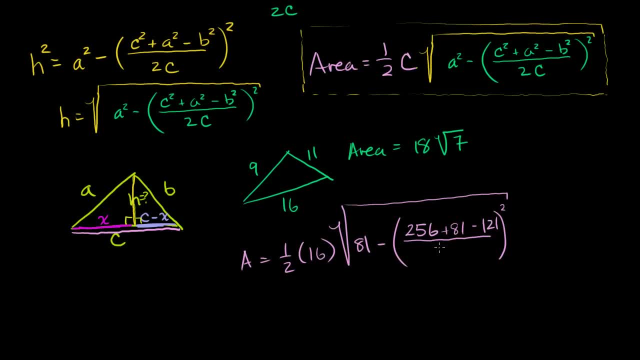 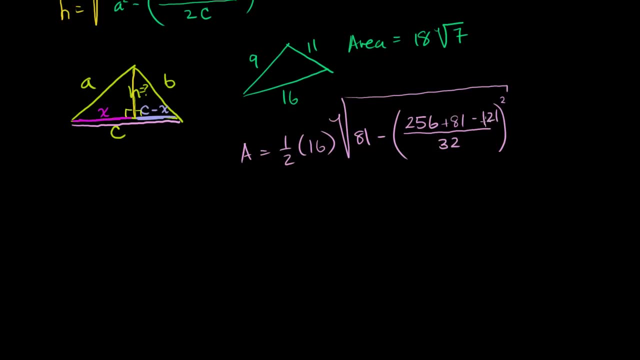 All of that over 2 times c, All of that over 32.. So let's see if we can simplify this a little bit: 81 minus 121, that is minus 40. So this becomes 216 over 32.. So area is equal to 1 half times a squared. 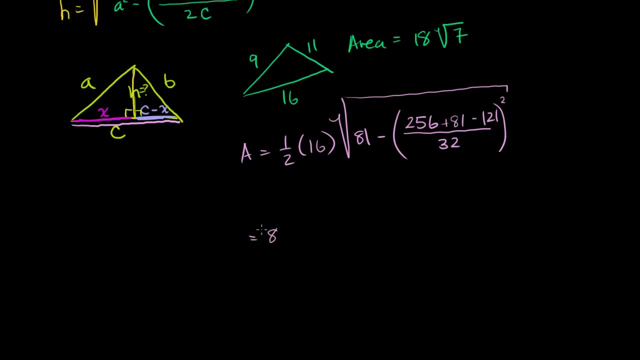 1 half times 8 is 8.. Let me switch colors: 1 half times 16 is 8 times the square root of 81 minus 256.. 81 minus 121, that's minus 40.. 256 minus 40 is 216.. 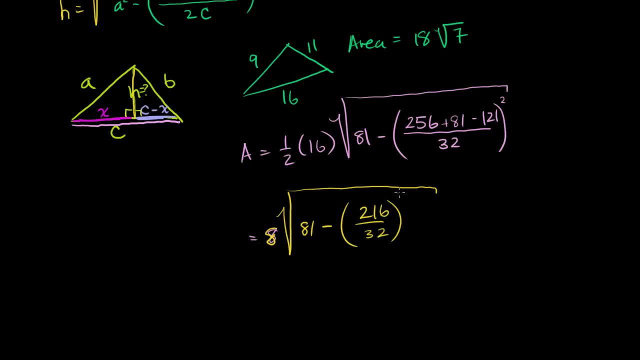 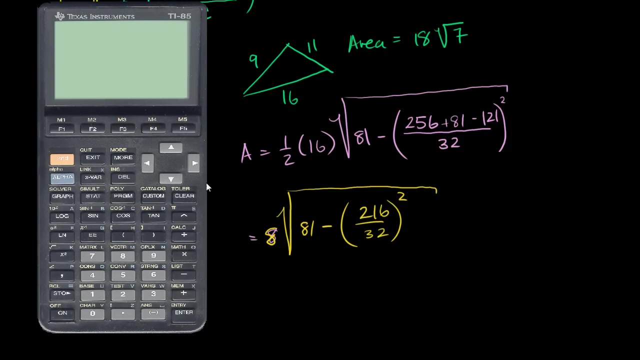 216 over 32 squared. Now this is a lot of math to do, So let me get out a calculator. I'm really just trying to show you that these two numbers should give us our same number. So if we turn on our calculator,